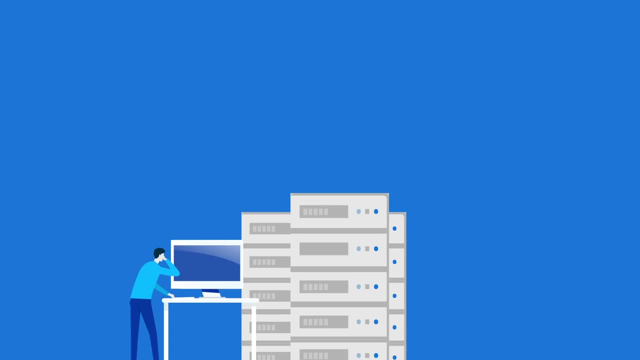 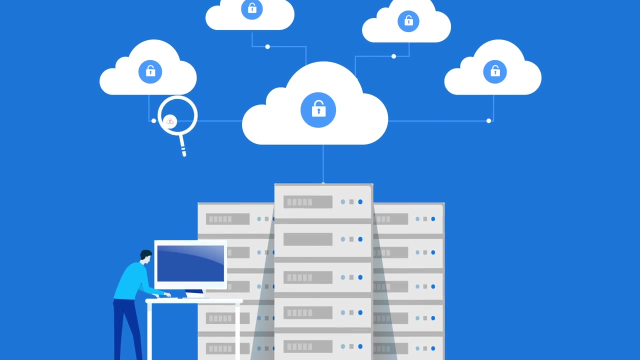 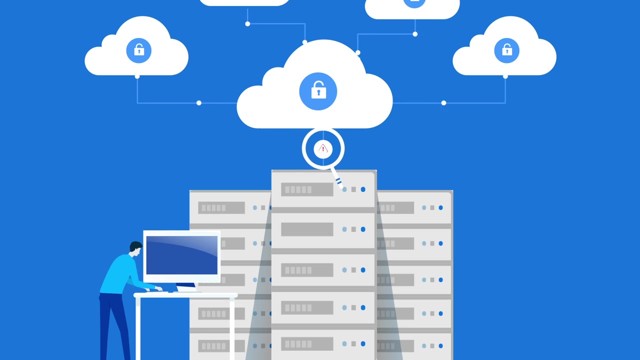 Intelligence, or CTI, plays such a critical role in cybersecurity. Think of it as an early warning system alerting you to the stealthiest and most damaging attacks out there. CTI gathers information about the digital and online dangers facing an organization. These dangers can be from a variety of sources across an organization's IT ecosystem. 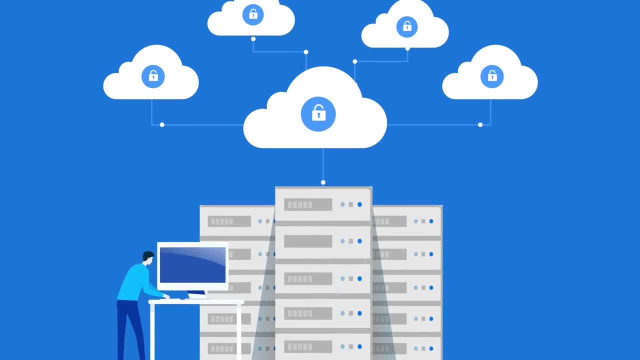 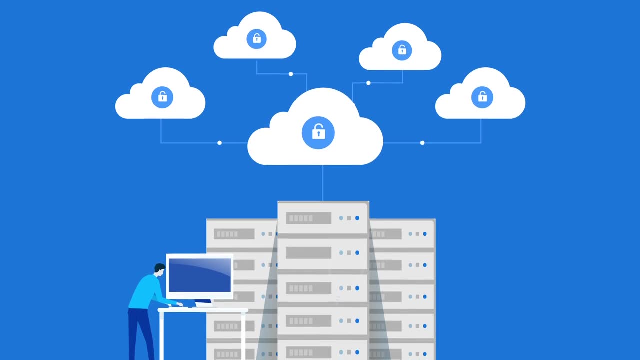 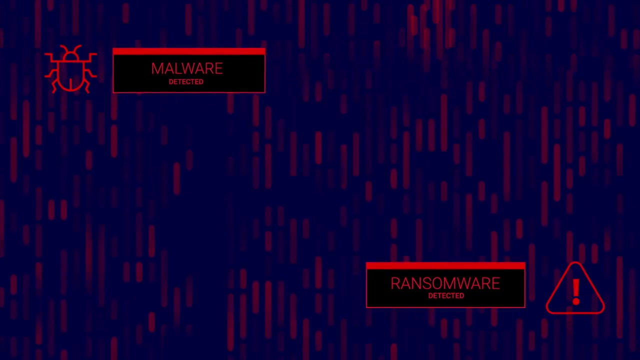 The information provided can be used to assess the severity of each threat and then form the basis of a strategy for prevention, protecting the organization from any expected dangers. Cyber attacks are on the rise. Analysts predict that the cost of damages due to malware and ransomware to businesses will reach $10.5. 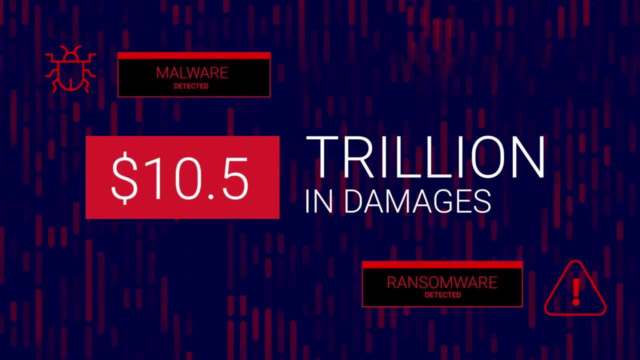 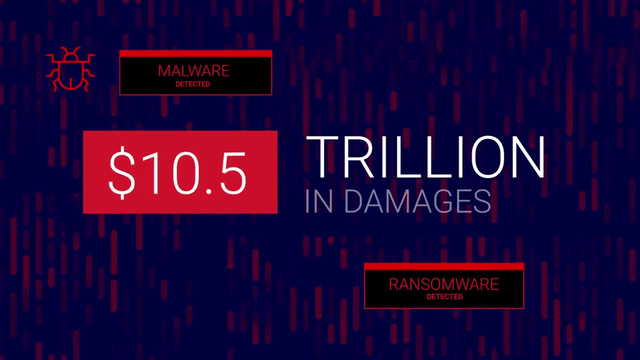 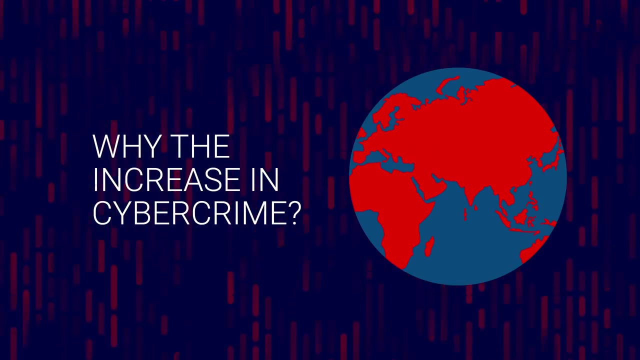 trillion by 2025, up from $3 trillion in 2015.. That's more than three times the costs in just a decade. It's more important than ever for organizations to do everything they can to thwart threat actors. Why the increase in cybercrime Attacks have become more sophisticated. 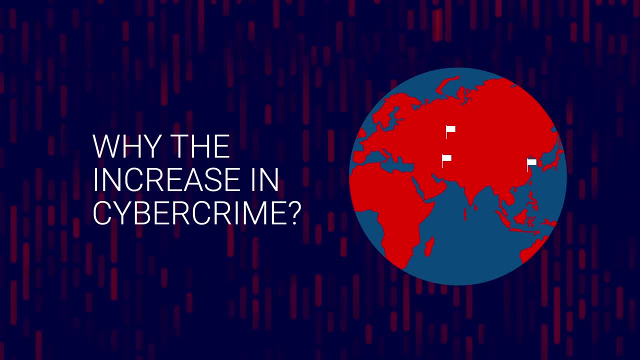 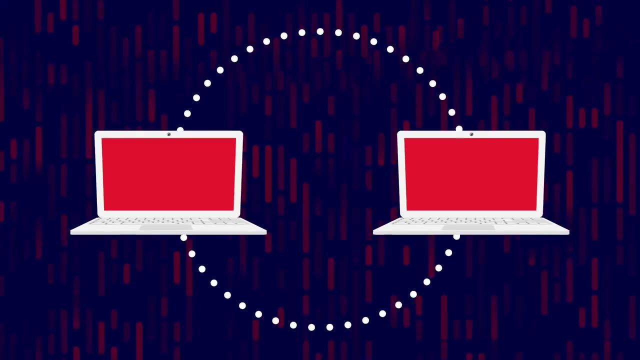 as the monetary rewards available have risen and even nation-states are weaponizing threat types such as ransomware to gain international political influence. Simultaneously, the proliferation of toolkits such as the Hive Group's Ransomware as a Service have enabled less technical 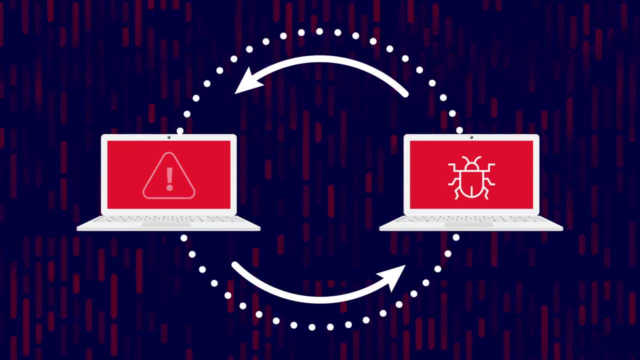 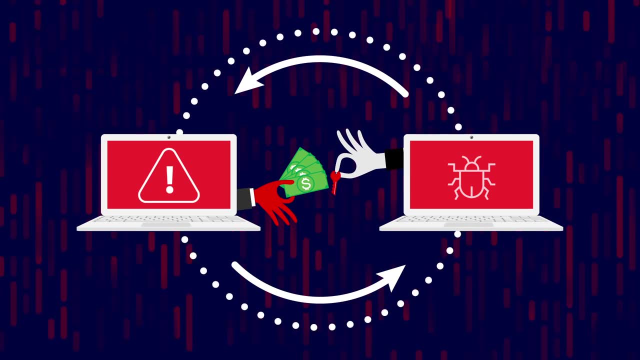 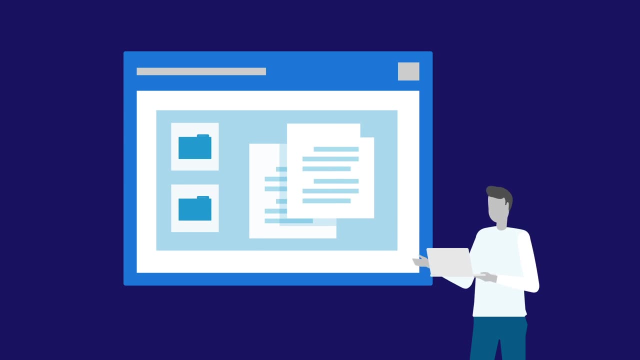 cybercriminals to rent cyberattack infrastructure for their own use, Or they can now buy access into a corporate system that has already been compromised by an initial access broker. CTI is a potent component of a proactive cyberdefense. It can help organizations assess. 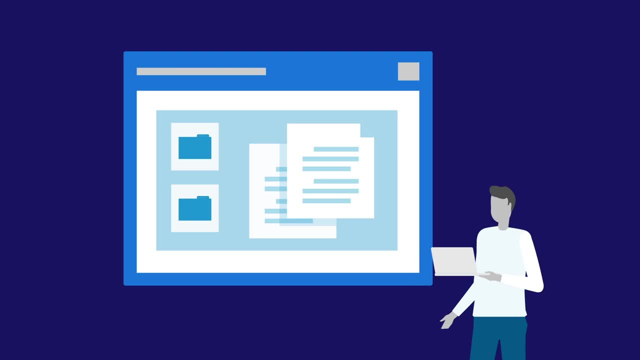 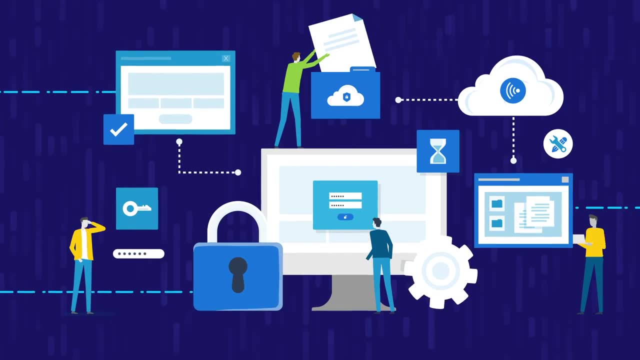 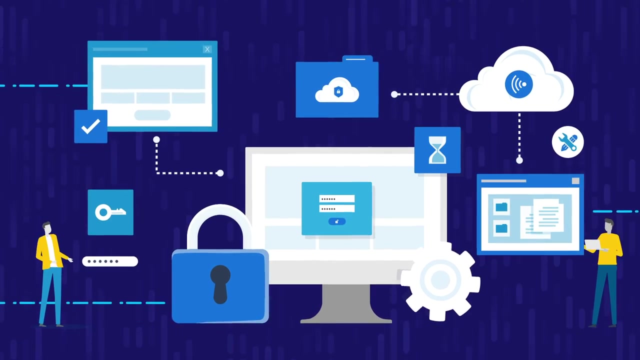 their risk of attack. CTI is tailored to their specific behavior, business focus and IT usage. By uncovering likely areas of threat, CTI shines a light on an organization's ecosystem and the threats it faces. This can form the basis of more data-driven decisions regarding risk and threat. 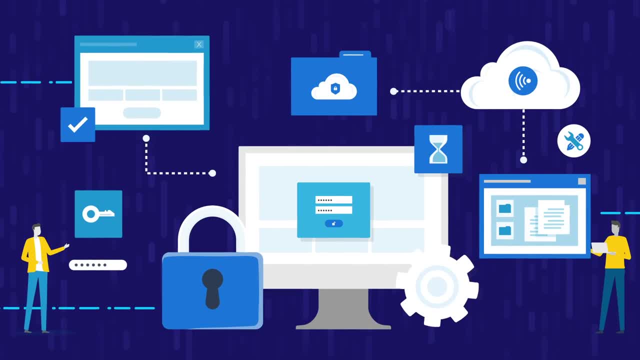 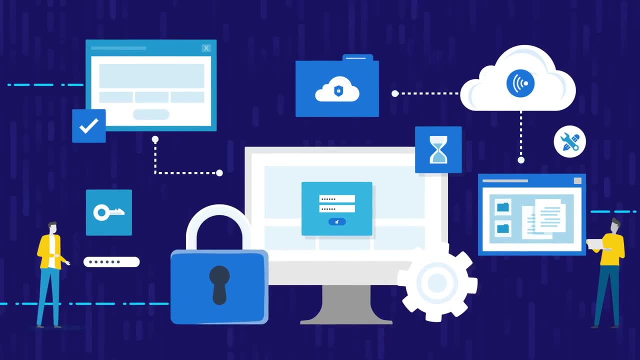 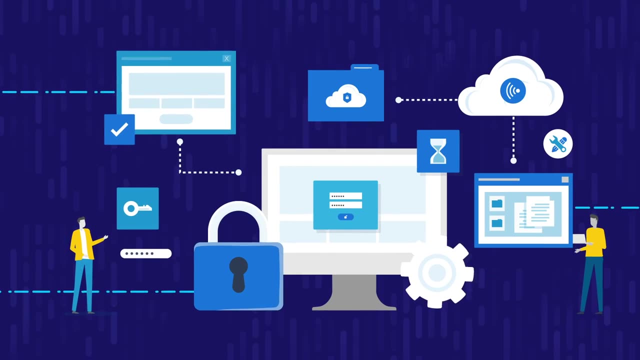 management Organizations can build a security strategy based on a solid understanding of the common tactics, techniques and procedures employed by threat actors. The result is fewer successful cyberattacks with defenses in place. CTI has been used to ward off more potential cyberthreats. greater resilience, more efficient. 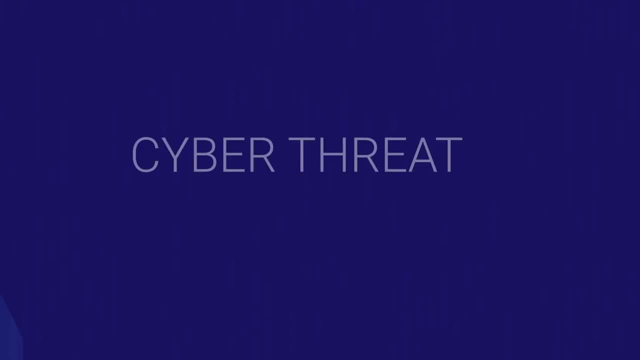 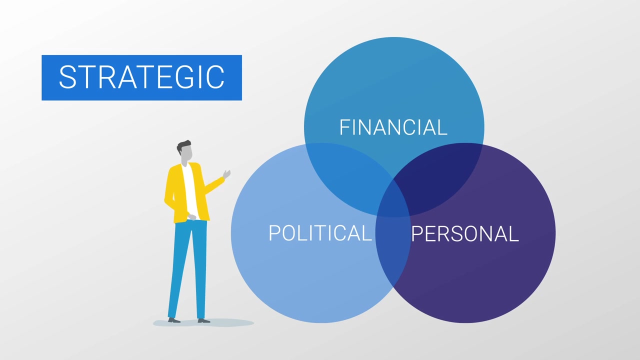 security and, ultimately, lower costs. There are four main categories of CTI. The first, Strategic CTI, is high level. It includes the overall threat environment, what could motivate attackers and potential impacts. Strategic CTI provides the basis for long-term. 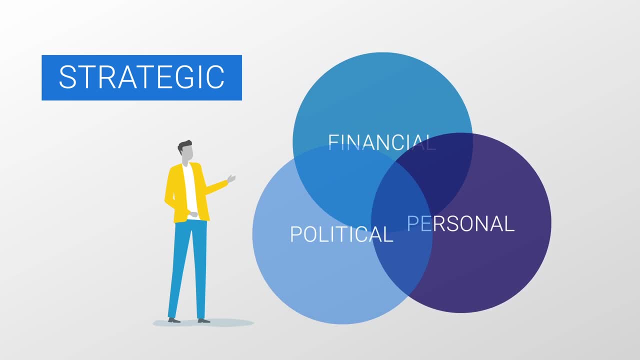 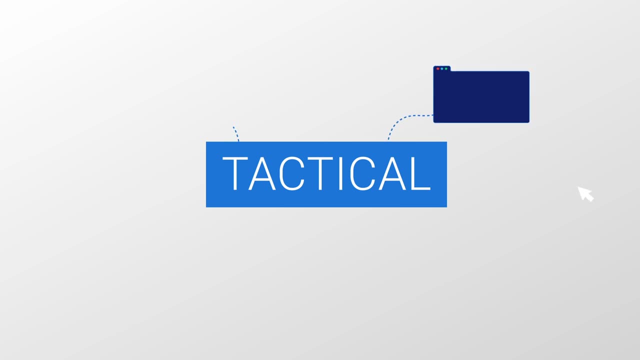 planning and helps organizations identify broader industry trends that may impact them. leaders can devise risk mitigation strategies. The second strategy is tactical CTI. This analyzes how the broader context affects an organization, specifically providing information about vulnerability types and how security teams can act to deliver defenses that mitigate them. The next two categories of 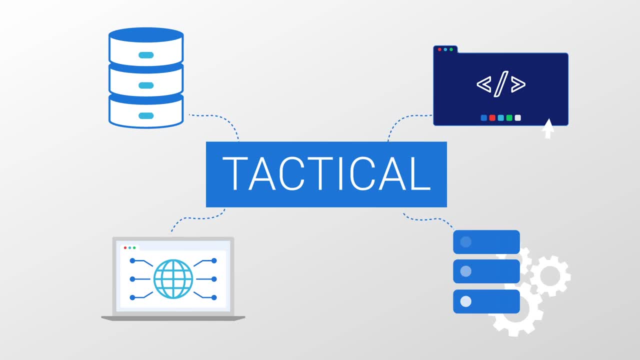 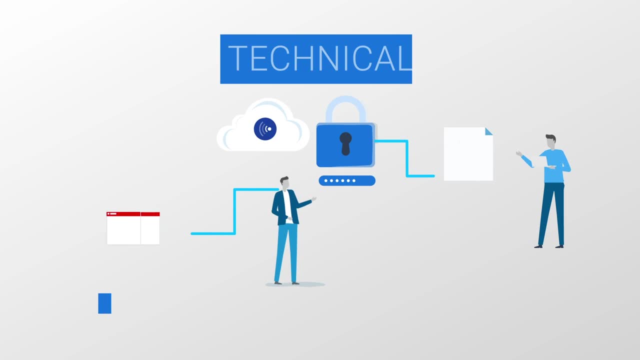 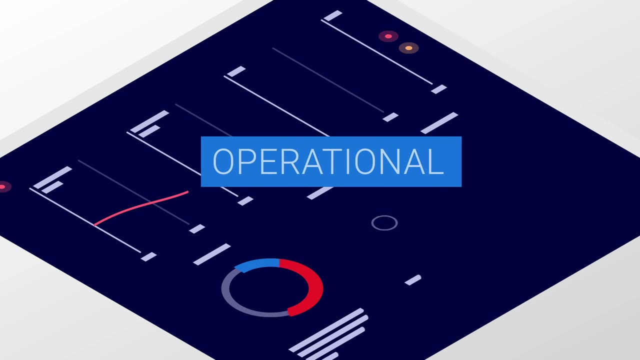 CTI- technical and operational- refer to the day-to-day methodology for preventing and dealing with cyber attacks. Technical CTI defines the indicators of attack with insights as to how to prevent the same or similar attacks. Operational CTI provides detailed, real-time knowledge about threats. This 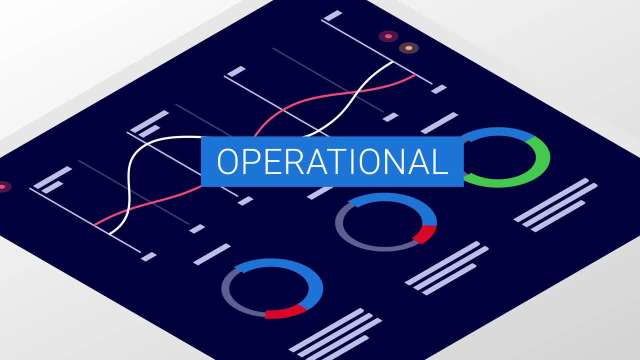 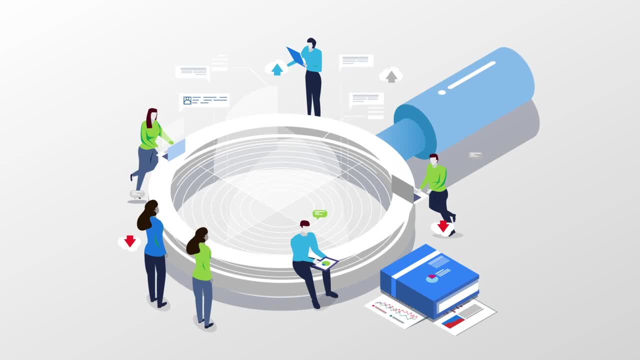 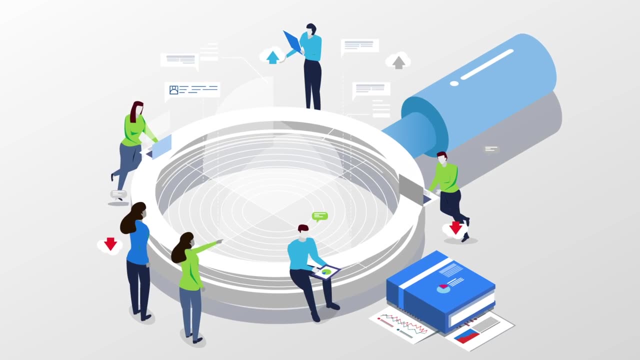 includes threat hunting and infiltration of threat actor communities. To implement CTI, an organization must first work out what needs protecting, including corporate assets and processes. Some of these may be more critical than others, Meaning an attack will have greater impact. Each asset can be prioritized for. 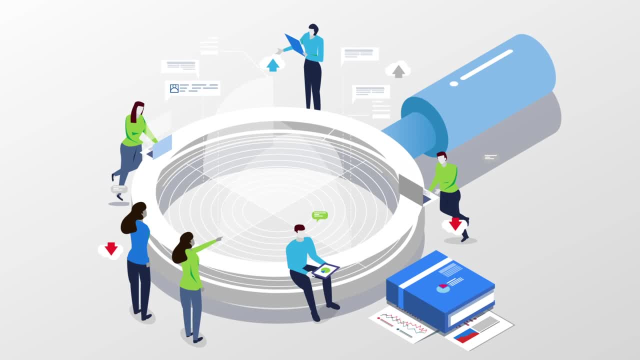 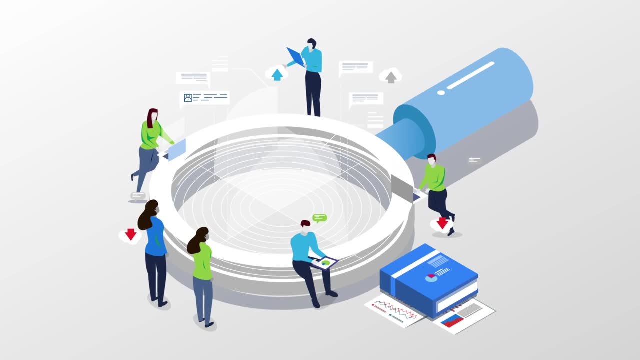 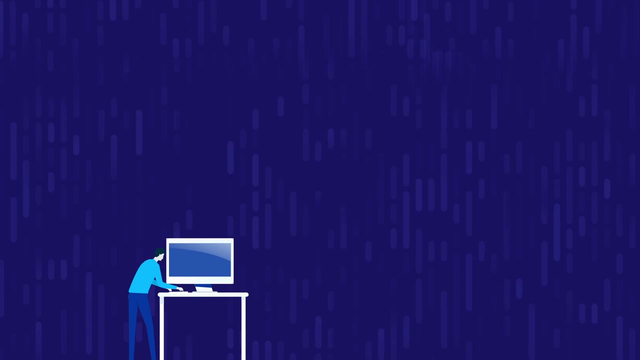 cybersecurity measures. During this initial phase, the organization looks at the motivations for attacks and which assets and processes could be vulnerable. This defines the attack surface and guides the types of CTI required to inform protection. Once the initial phase is complete, the CTI process involves: 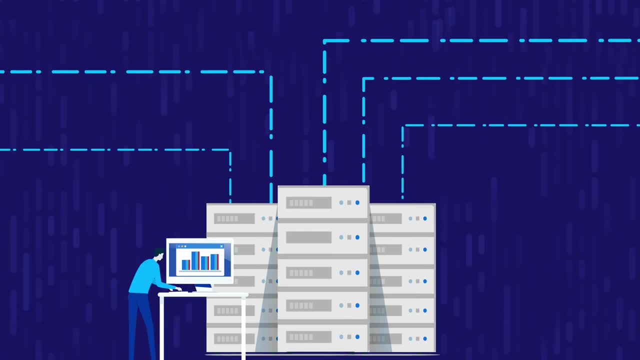 collecting raw information from internal and external sources. These could include the logs from antivirus software and website traffic reports, industry updates from cybersecurity specialists and other forms of monitoring data. This data is then processed into an organized form. The processing is likely to employ advanced techniques such as artificial. 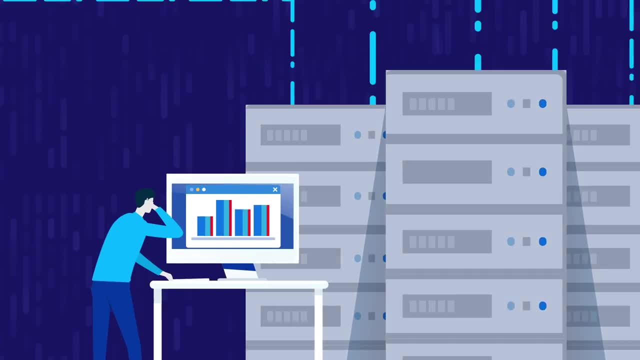 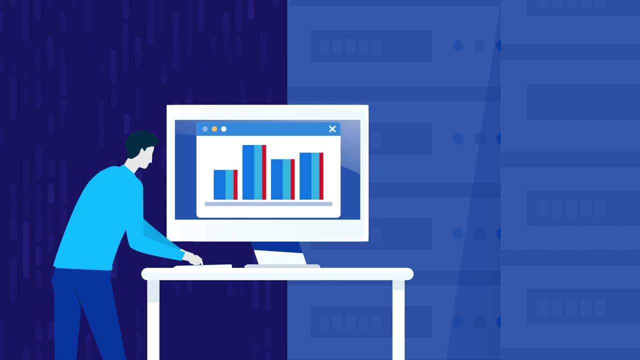 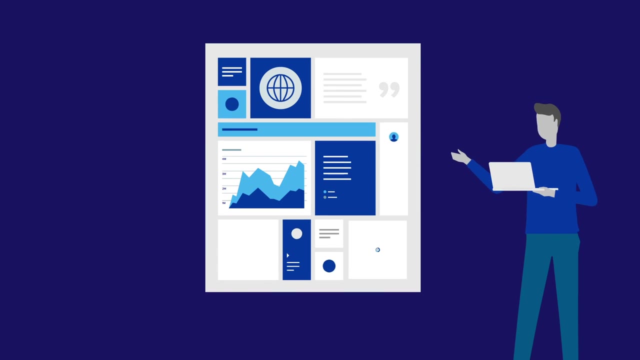 intelligence and machine learning to assist with structuring. Once the information is processed, security experts can analyze it using their skills and knowledge. to add context, This results in detailed insights and defensive plans. These core insights and the actions that can be taken against threats can then be disseminated to stakeholders. This forms their guide for